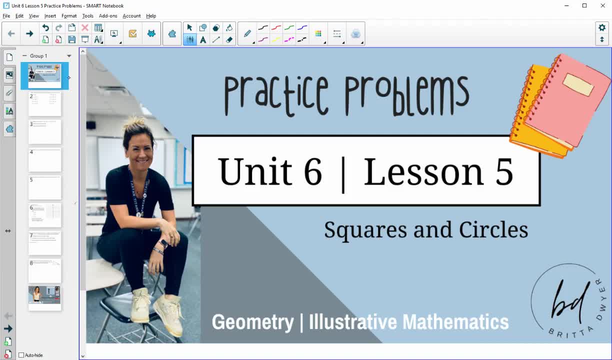 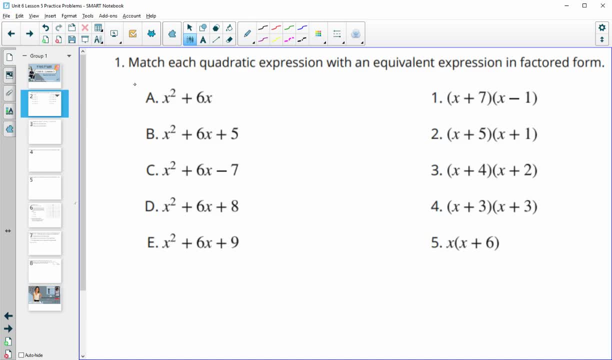 In this video we're going to take a look at the Unit 6, Lesson 5, Practice Problems for Geometry. Number 1 asks us to take each quadratic expression and match it to its factored form. So this first one. we see that both terms have an x in them, so we'll be able to factor that out. 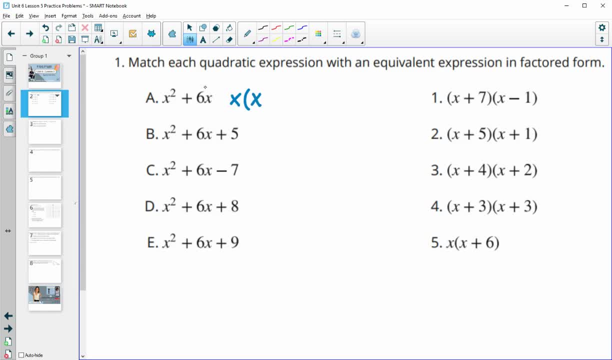 So when we do x squared divided by x, we get x, and 6x divided by x gives us 6.. So we can just distribute that x out and we end up with number 5.. So a goes with number 5.. 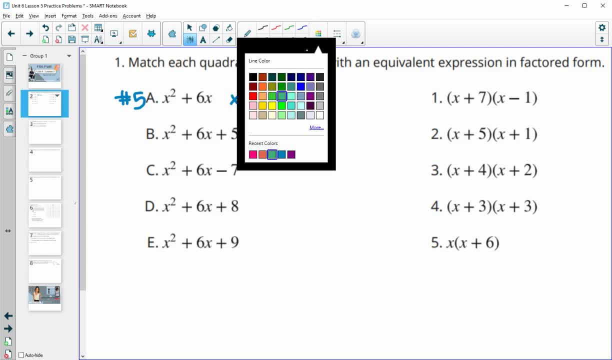 Then we get into trinomials, so quadratics with three terms, So we can take this final number here and see what numbers multiply to 5 and add to 6.. And so the numbers that add to 5, or sorry, multiply to 5 and add to 6,. 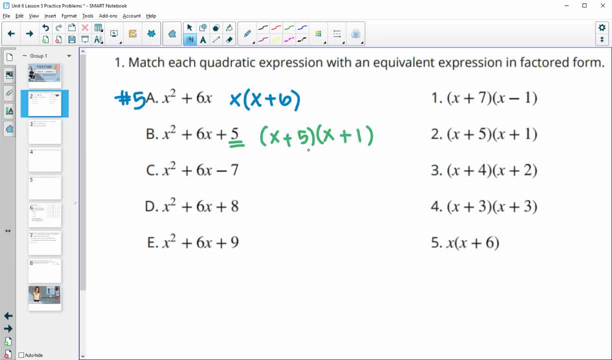 are 5 and 1.. So in this middle term you'd get 5 times x, which is 5x, and then you'd get 1 times x, which is 1x, 5x, and 1x adds to that 6x, and then 5 times 1 gives you the 5 at the end. 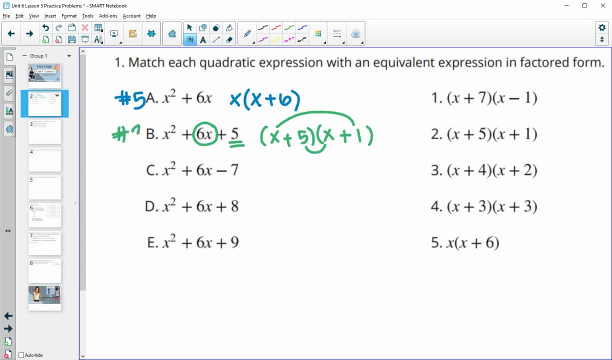 So this one is number 2.. Next one: your final term is negative 7.. So now they need to multiply to negative 7.. So 1x is negative 7.. So 1x is negative 7.. So 1x is negative 7.. 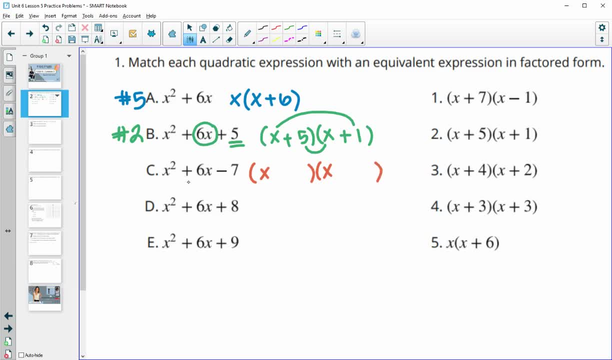 So 1 is going to be positive and 1 is going to be negative, And then they need to add to positive 6.. So we know that we're going to have a 7 and a 1, since that's the only numbers that multiply to 7.. 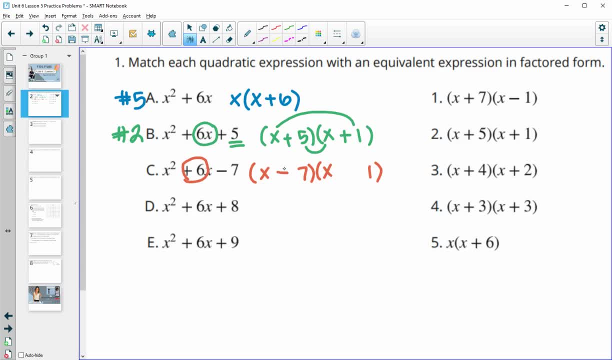 And then we want the 6 to be positive. So we're going to need a positive 7 with a negative 1, because that's going to give us positive 7x and negative 1x for the 6x in the middle. 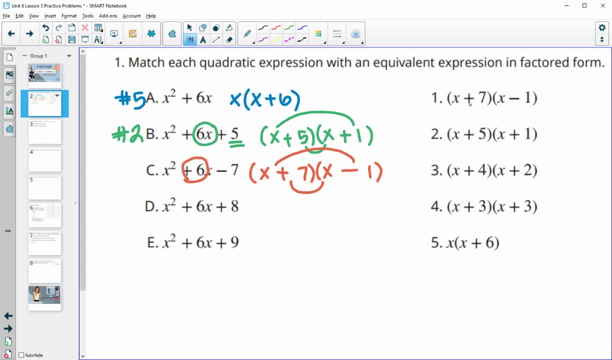 And then positive 7 times negative. 1 gives us that negative 7.. So that's number 1.. Next one: our final term is 8. So now we want the factors that multiply to 8 and add to 6.. 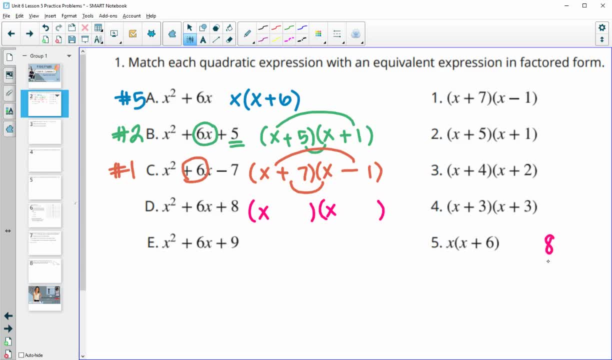 So 8's not a prime number, so we're going to have some options here So you can write out the factors of 8.. So 1 and 8, or 2 and 4.. So which of those adds to 6 is the 2 and the 4.. 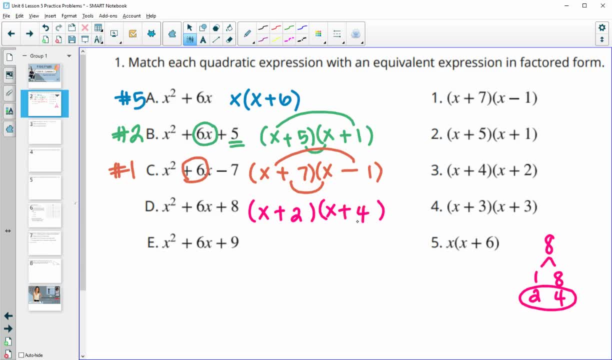 So we'd have to have a positive 6.. We'd have to have a positive 2 and a positive 4, so that it multiplies to positive 8 and adds to that positive 6.. And so then that's going to be number 3, even though I have it written backwards. 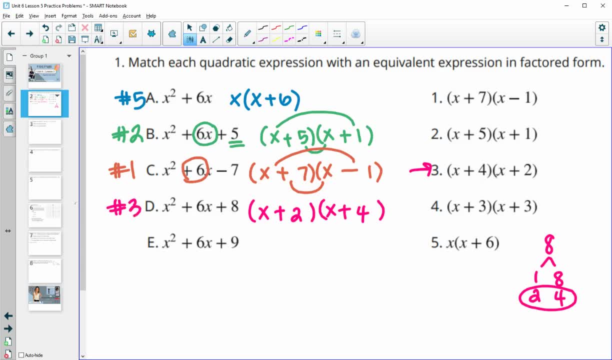 It doesn't matter, since it's multiplication. So you can either have x plus 4 first or you can have x plus 2 first, And then that leaves number 4 left over for e. Numbers that multiply to 9 and add to 6 are 3 and 3.. 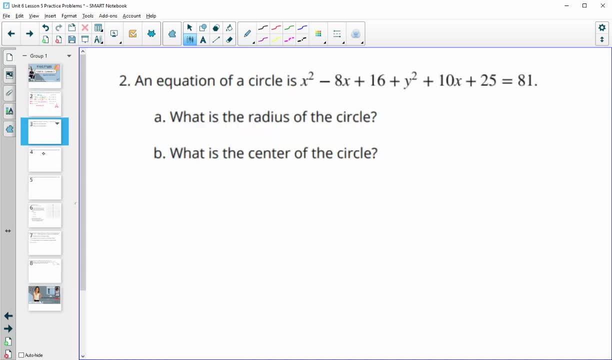 Number 2,. an equation of a circle is written like this: What is the radius of the circle and what is the center? So we've got two different parts here. We've got this x part and then we've got the y part. 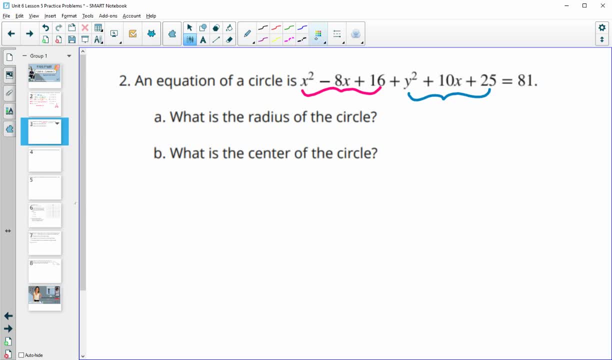 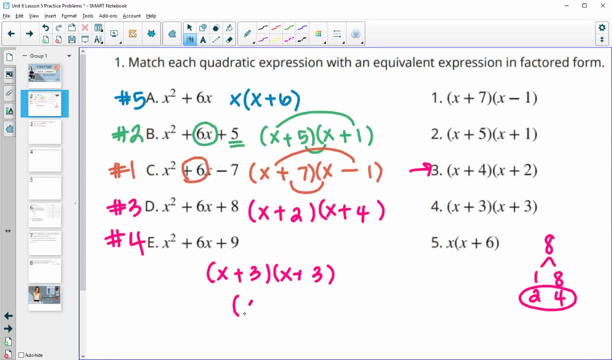 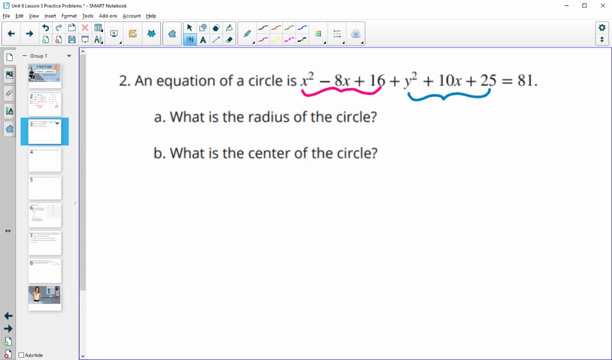 which are perfect square trinomials, meaning that they will factor to the same number, just like this where these are both x plus 3.. So we could write it as this: x plus 3 squared. So right here, the numbers that multiply to 16, that add to negative 8,. 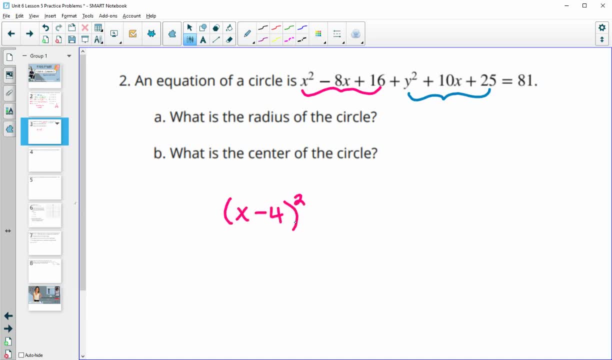 that's x minus 4 squared, because negative 4 times negative 4 is positive 16, and negative 4 plus negative 4 is that negative 8.. And then the y part gives us y plus 4, so the 5 times 5 gives us 25,. 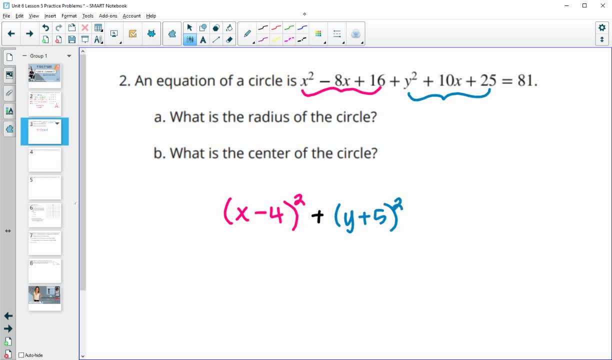 and 5 plus 5 gives us the 10 in the middle. so y plus 5 squared And then that's equal to the 81. still, And remember, 81 is our radius squared. so what number squared gives us 81 is 9.. 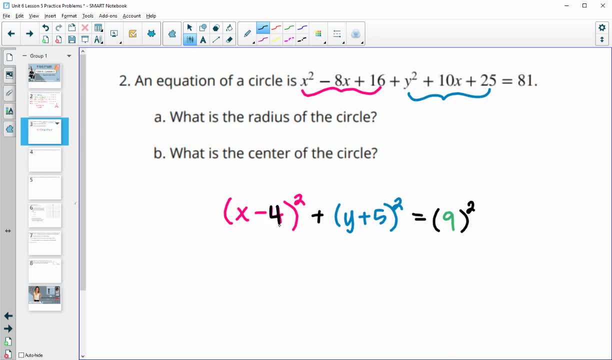 So our center here is going to be the number we subtract from our x, so that's going to be 4.. And then the number we subtract we subtracted from y, so we subtracted a negative 5 from y, So our center is 4 negative 5,. 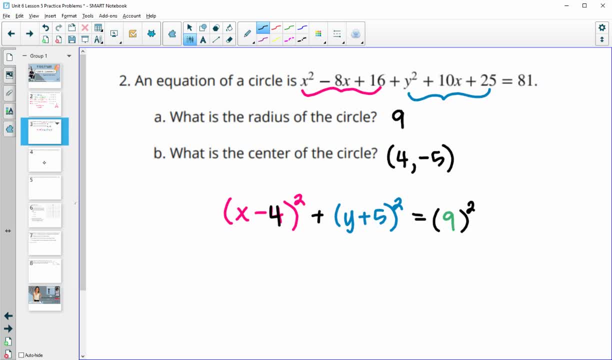 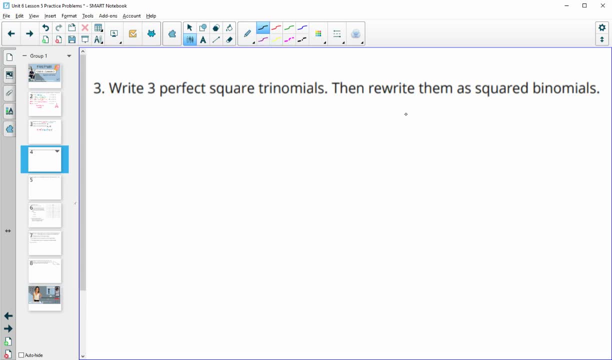 and then our radius is 9.. Number 3, write 3 perfect square trinomials, then rewrite them as squared binomials. So we're just making up our own here. so you can make up whatever you want. You do need the last term to be a perfect square. 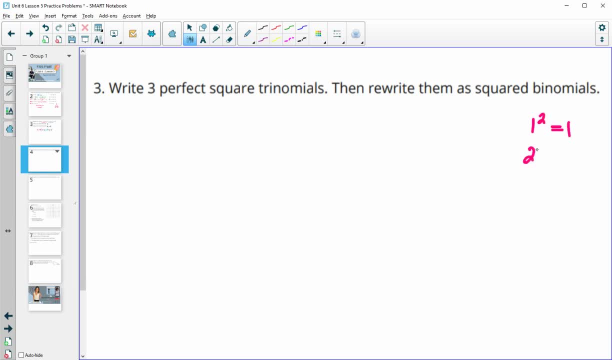 so, when we're thinking about perfect squares, 1 squared is 1,, 2 squared is 4,, 3 squared is 9.. So these numbers, these perfect square numbers, you're going to need at the end. So you need to use a perfect square number. 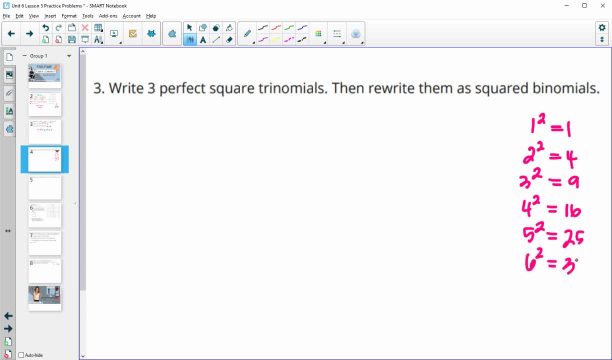 Now, these are just the first few. You can certainly use other ones as well. So if you were going to do something like that, so if we were going to use 16 as our final number, so we'd have x squared at the end. 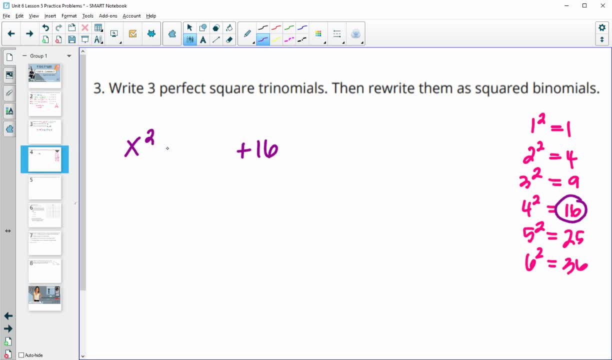 and we'd have 16, and 16 is 4, so this middle term we would want to have as 8x, so 4 plus 4, or we could have it as negative 8x, because negative 4 times negative 4 is 16,. 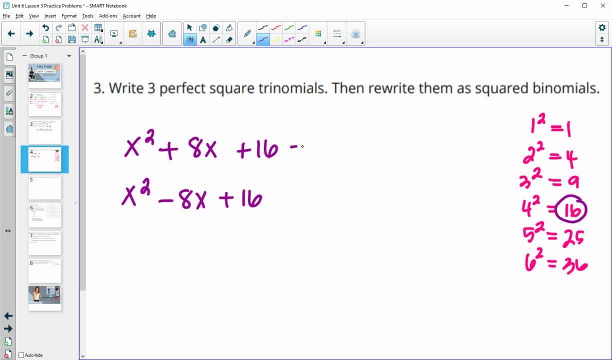 and negative 4 plus negative 4 is negative 8.. So then, as a perfect square binomial, this one would be x plus 4 squared. This one would be x minus 4 squared. So you want to make sure that you have a perfect square. 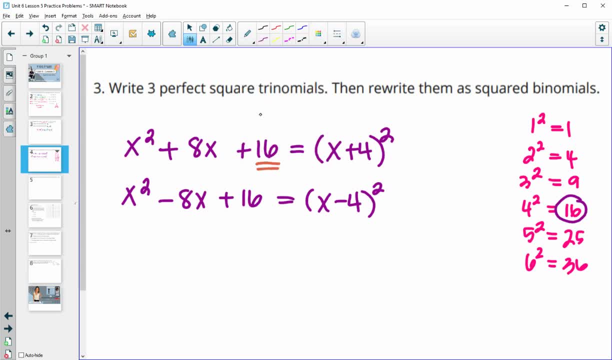 and you want to make sure that this end number is your number squared and that this middle number is that number times 2.. So then another one we could do if we wanted to pick, like: let's do the middle, let's do the end number as 9 squared, so 81.. 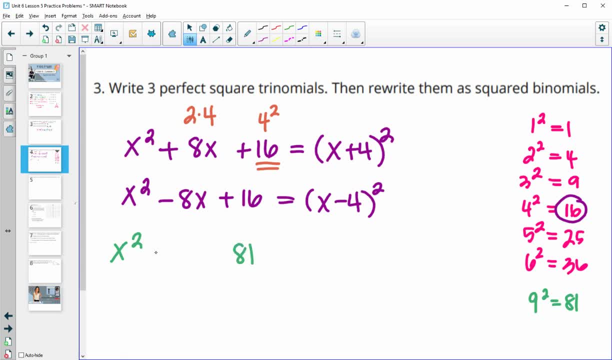 So then we could have 81 at the end. So then this middle number would need to be 9 plus 9, or 18. And it could be negative 18 as well. So this is four different perfect square trinomials for you. 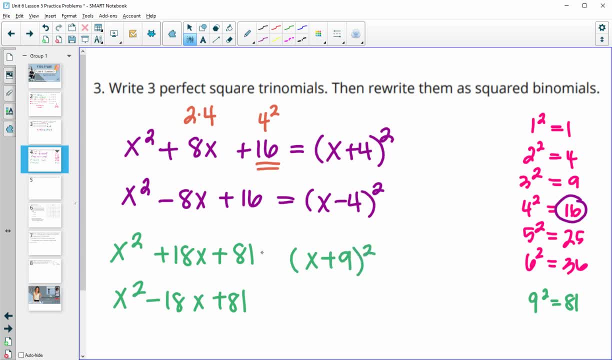 So this one would be x plus 9,, since 9 times 9 is 81, and 9 plus 9 is 18.. Or this one would be x minus 9 squared, so that we get that negative 18x in the middle. 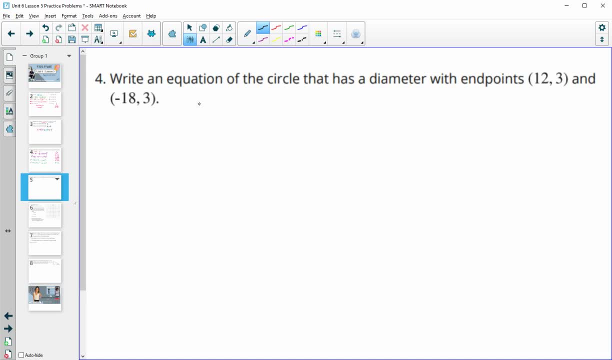 Number four: write the equation of a circle that has a diameter with these two end points: okay, So the diameter right goes across the circle, And so we need the center. So this one is at negative 18,, 3,. 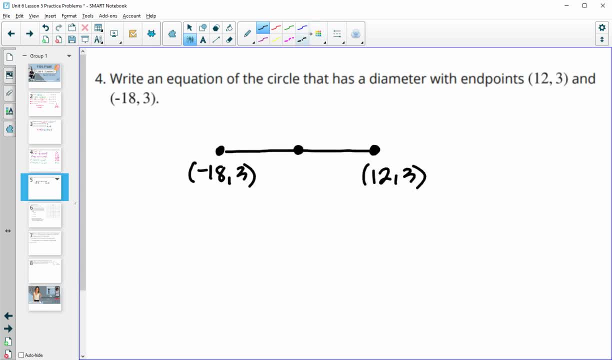 and this one is at 12,, 3.. And we notice, hopefully, that these y values are both the same, So it's at the same height. So I know that the y coordinate here will be a 3.. Okay, because it's gonna stay the same. 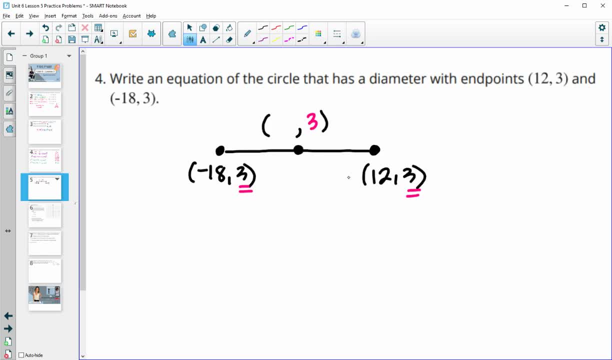 We're looking for the middle number. So now we just have to find the middle of negative 18 and 12.. And so you find the middle by doing the average- So negative 18 plus 12, and then dividing it by 2.. 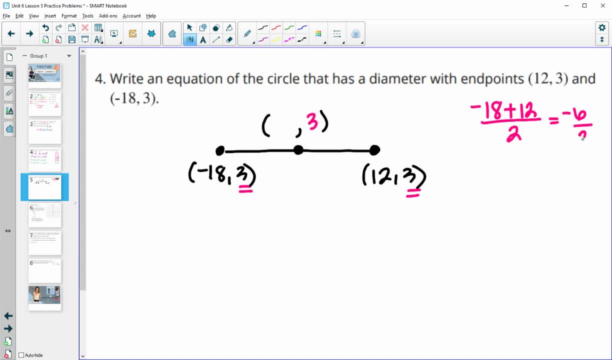 So negative 18 plus 12 is negative 6, divided by 2 gives you negative 3.. And then I like to just check. So negative 18 to negative 3 is 15 away, so plus 15.. And then 12 to negative 3 is also plus 15, just to make sure that it's in the center. 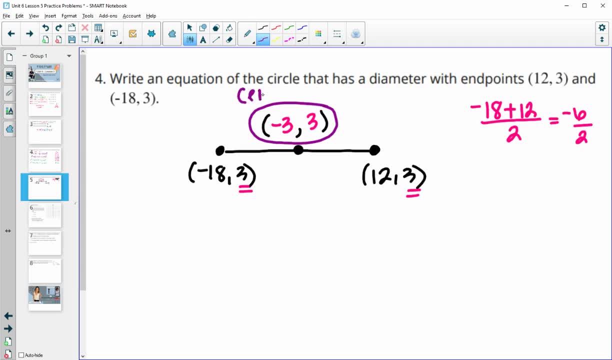 So this is your center of your circle, And then we need the radius, which is actually that 15 that we just talked about, because that's how far the center is to the edge would give us 15 units. So now you just want to plug this into your circle equation. 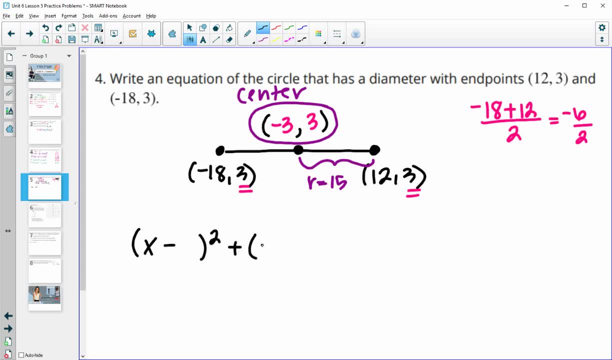 which is x minus the x-coordinate of the center squared, plus y minus the y-coordinate of the center squared, equals your radius squared. So your center point okay. your x-coordinate of your center is negative 3.. So we'll plug in negative 3 here. 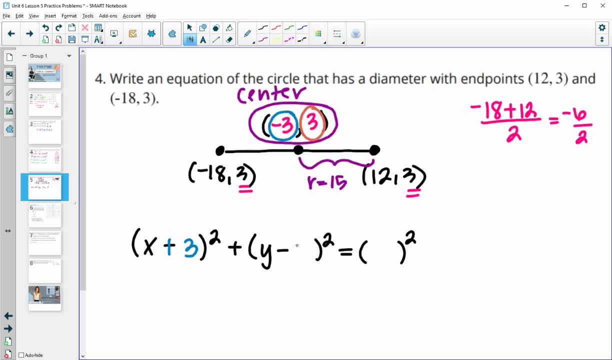 And then your y-coordinate of your center is 3.. And then our radius is 15.. So that was That would be your circle equation. You can certainly multiply out the radius if you want. So it's going to be x plus 3 squared plus y minus 3 squared. 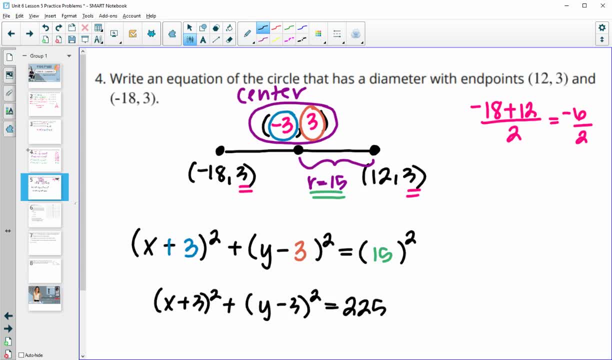 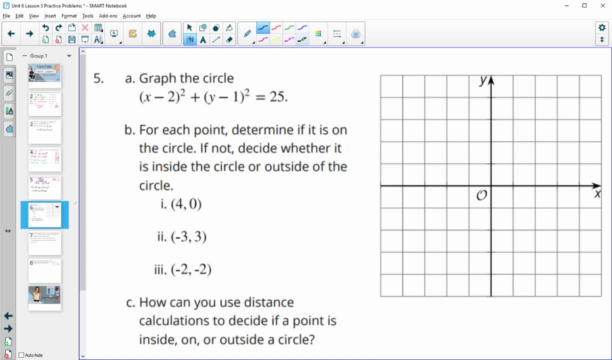 And then 15 squared is 225.. So you can write it as either of those Number five graph this circle, And then we're going to do some stuff with it. So first we need the center. Okay, so the center here is going to be 2.. 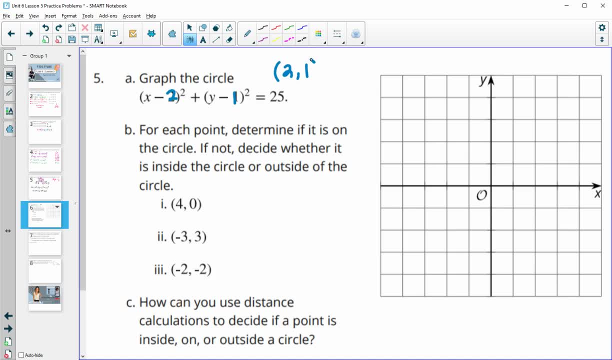 1.. Okay, so we subtracted 2, and we subtracted 1 from the x and the y, So the center point is at the point 2, 1.. So here's our center, Then our radius. So this is our radius: squared is 25.. 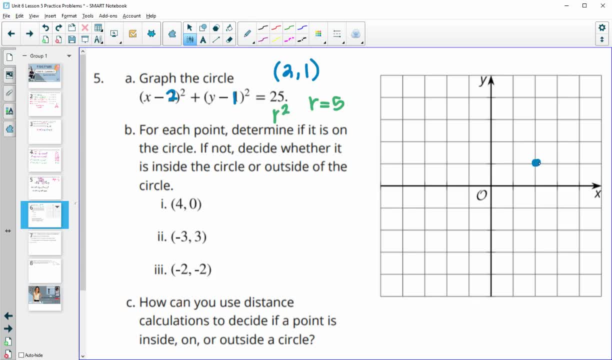 So our radius is 5.. So we're going to want to count out 5 from each of these. Okay so, 1, 2,, 3, 4, 5.. 1,, 2,, 3, 4.. 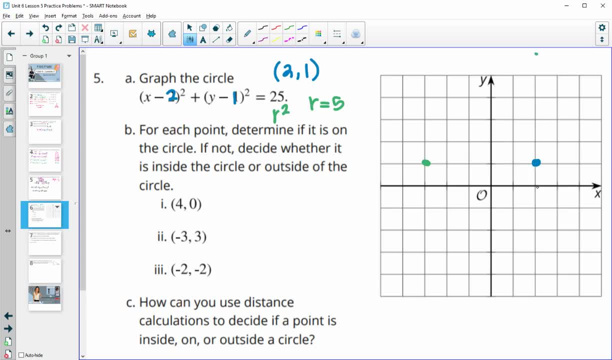 And that's going to go off. This one's going to go off. 1, 2,, 3,, 4, 5.. So you could have changed this and counted by twos if you wanted. I'm not going to, because I can just use this circle tool to get my circle drawn here. 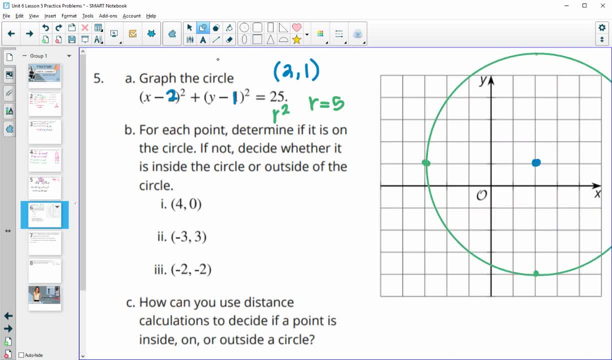 So just go out to a radius of 5.. Now you might have wanted to change it to twos, so you can try and look and see if these points are on it. However, I'm actually going to plug each of these points Into my equation to prove whether or not they're on the circle. 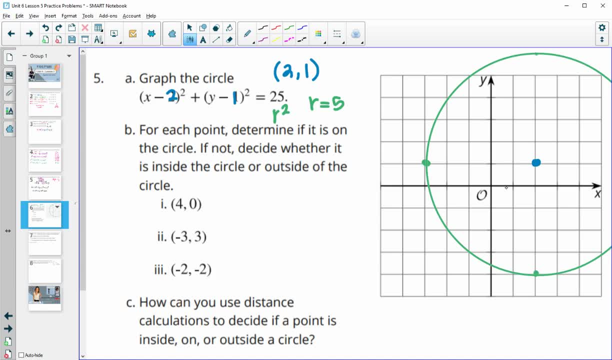 So this point: 4, 0. And you could look 1,, 2,, 3,, 4. It's clearly not Okay because it's on the inside of the circle And so we know that that one's not. 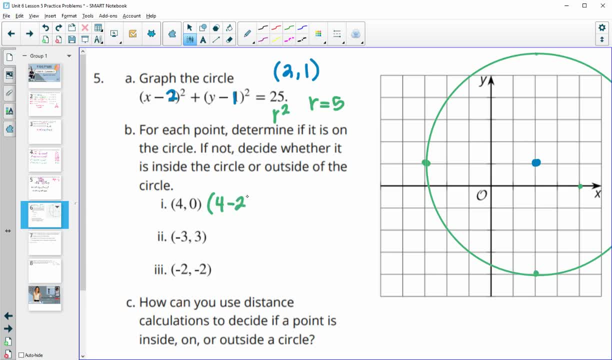 But we can also plug it in here. The x is 4.. So 4 minus 2 squared. So I'm just plugging it in, And then the y coordinate is 0.. So 0 minus 1 squared, And that should. 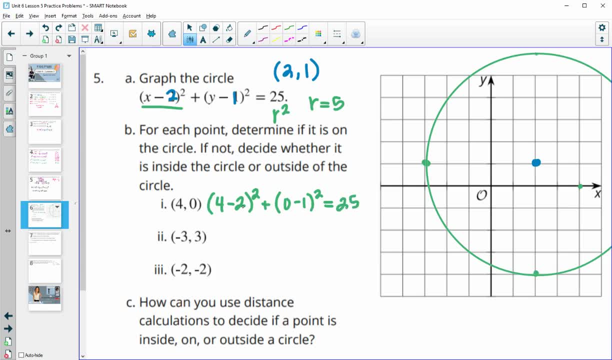 Equal 25 if it's on our circle. Well, 4 minus 2 is 2 squared. And then this is negative 1 squared 2 squared is 4.. Plus negative 1 squared is 1.. That does not equal 25.. 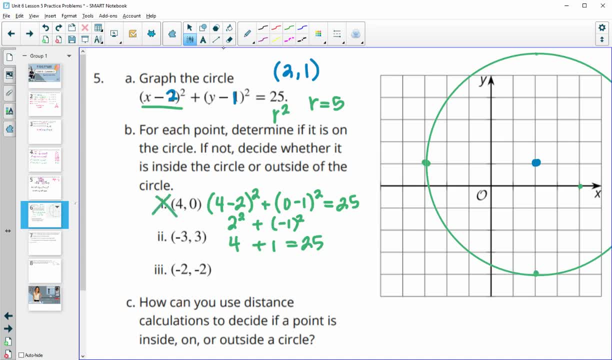 That only equals 5.. Okay, so this is bad. Okay, so that one is not on the circle. Then Let me see, I'm just going to move this up Here. Okay, so then we can plug in these ones into the circle equation as well. 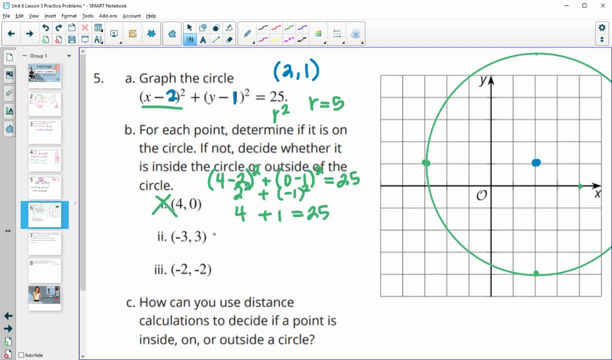 And so this one, we've got negative 3 minus 2.. So negative 3 minus 2 is negative 5 squared, And then we'll do 3 minus 1.. Okay, so we're plugging this into the y coordinate. 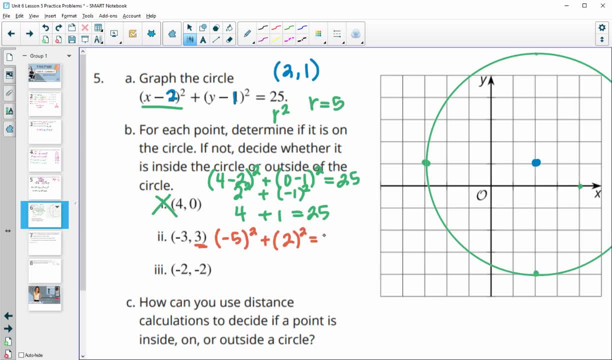 So 3 minus 1 is 2 squared, So then 25. Plus 4. Because this is 25 when we square it Plus 4 does not equal 25.. So this one is not on the circle either, And you can see that here at negative 3, 3 would be inside of our circle as well. 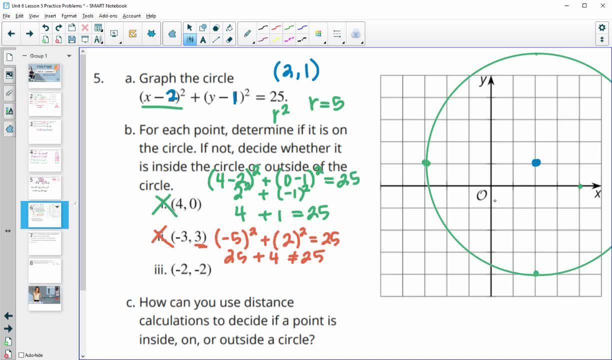 Oops, that's not negative 3, 3.. That's 3, 3.. Okay, so negative 3, 1, 2, 3.. Negative 3, 3 is outside of our circle, And then you can plug in this last one. 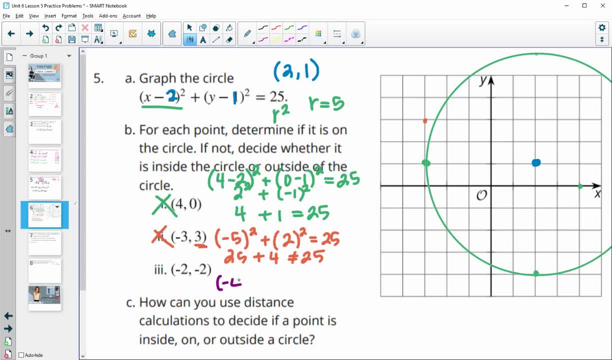 So then negative 2 minus 2 is negative 4. 4 squared. And then negative 2 minus 1 is negative 3 squared: Negative 4 squared is 16.. Negative 3 squared is 9.. 16 plus 9 is 25.. 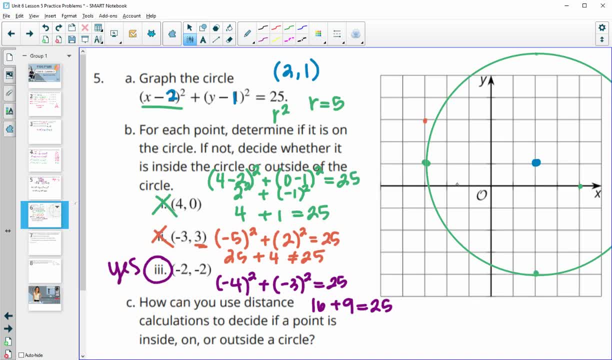 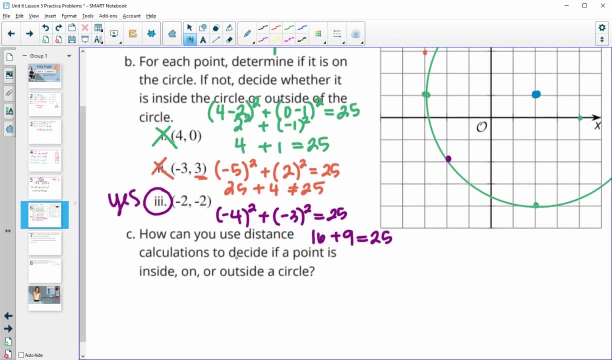 So this one is on our circle And you can go to the point negative 2, 2 and see that it looks like it crosses there as well. So how can you use distance calculations to decide if a point is in the circle? So you can use distance calculations to decide if a point is inside, on or outside of the circle. 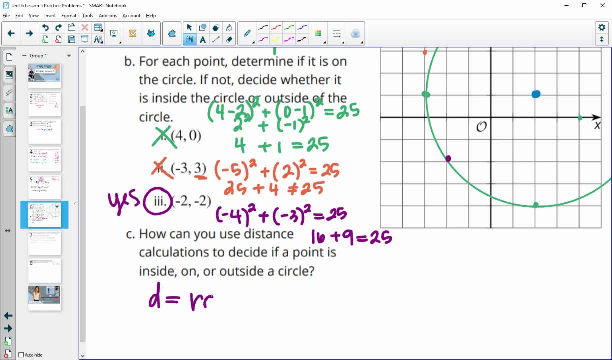 So if your distance is equal to the radius, then it's going to be on the circle. If your distance is greater than the radius, then it's going to be outside the circle. So, like this one where the distance was 29, that's outside of the circle. 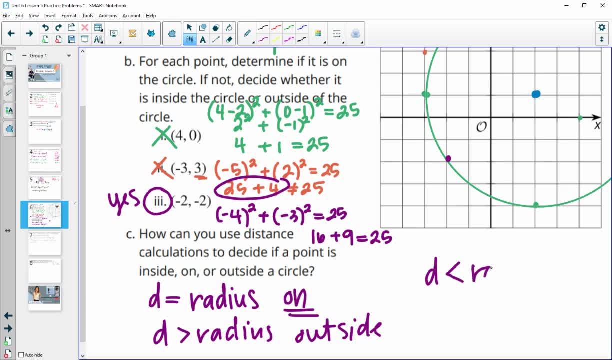 Or if your distance is less than the radius, okay then the point is going to be inside, And we saw that with this one, where the distance was 5. Well, really, square root of 5., But that's less than the radius. 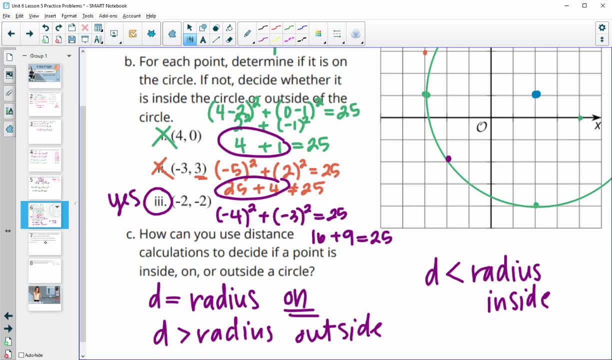 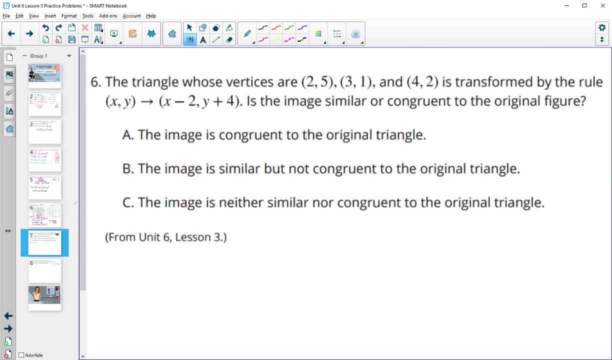 So that one's going to be inside the circle Number 6, the triangle whose vertices are 2, 5, 3, 1, and 4, 2 is transformed by this rule. Is the image similar or congruent to the original figure? 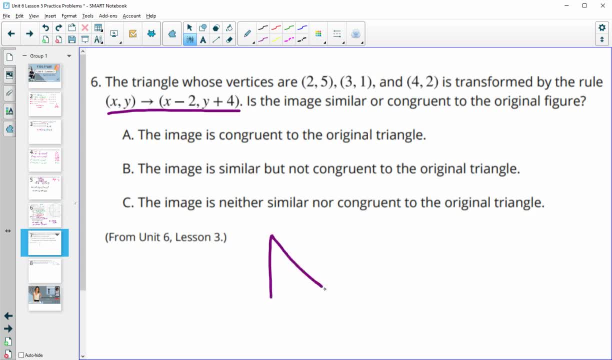 So, remember, when we add and subtract, that's just taking the triangle. Okay, so this was our random triangle. That's just taking this exact same triangle and just moving it to the left, 2 and up, 4. So it doesn't change the size. 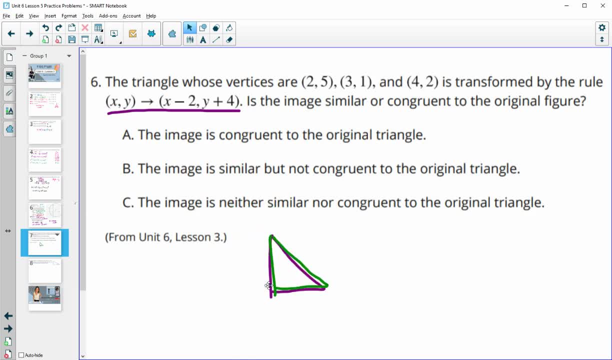 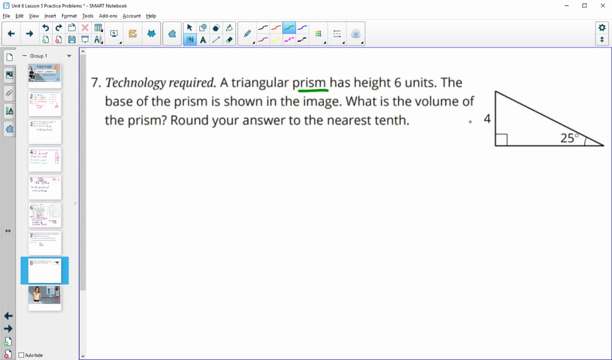 It's just translating it okay around your graph, So the image is going to be congruent to the original triangle. Number 7,: a triangular prism has a height of 6 units. The base of the prism is shown. What is the volume? 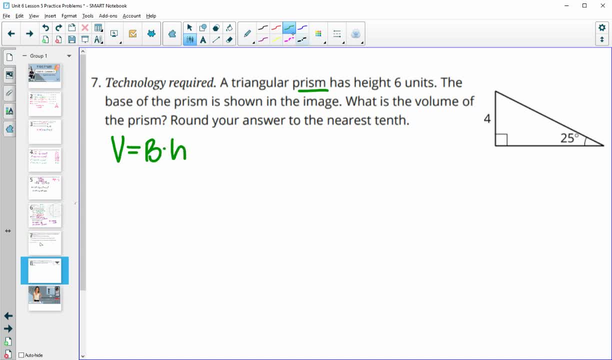 So, remember, volume is area of the base times the height, And they give us our height here. Remember, a triangular prism is just going to be like this: where your base is, our triangles, And it's just three-dimensional. So this is what we're doing. 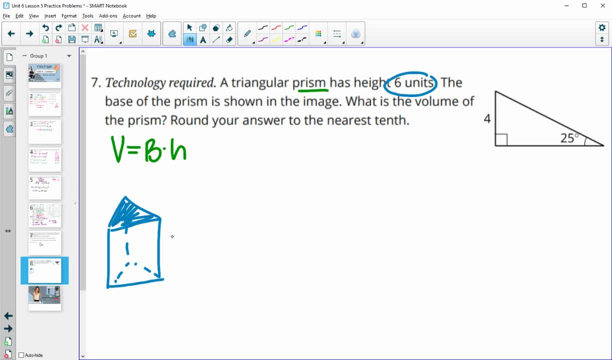 This base, right here is this triangle. So we have the height is 6.. Now we just need to calculate the area of this base. So to do the area of a triangle you need to do the base times the height divided by 2.. 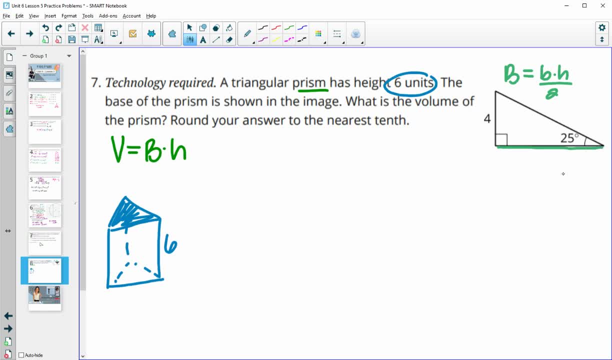 So we have the height of this triangle. We just need this base length, And so we're going to have to use trig for that. So we've got the angle. 4 is the opposite side. The side we're looking for is the adjacent. 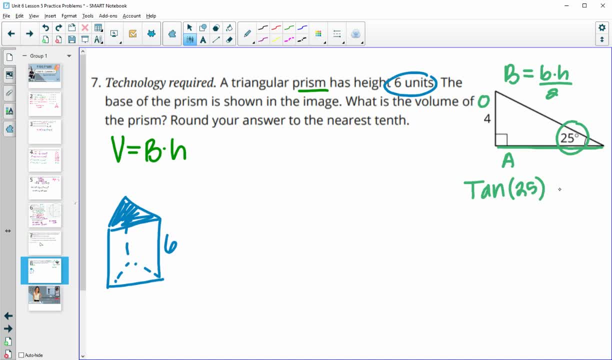 So that's going to be a tangent function. So we're going to do: tangent of 25 equals the opposite side over the adjacent side. So then we'll multiply both sides by X And then we'll divide by tangent of 25 to both sides. 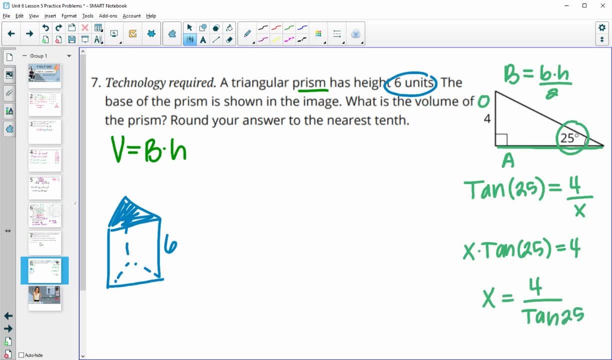 And then that's what we'll type into our calculator is 4 divided by the tangent of 25.. And that gives us 8.58 for that length, Whoops, 8.58.. So then, when we go to calculate the area of that base, 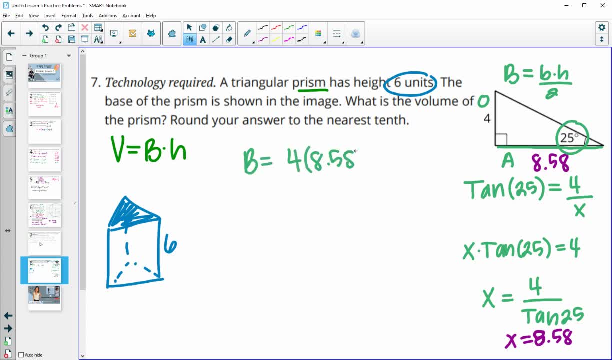 we'll be doing 4 times 8.58 and dividing that by 2. And we'll get a base area of 17.16.. And then we have this height here of 6 when we go to actually calculate the volume. So our volume is going to be area of the base times the height.